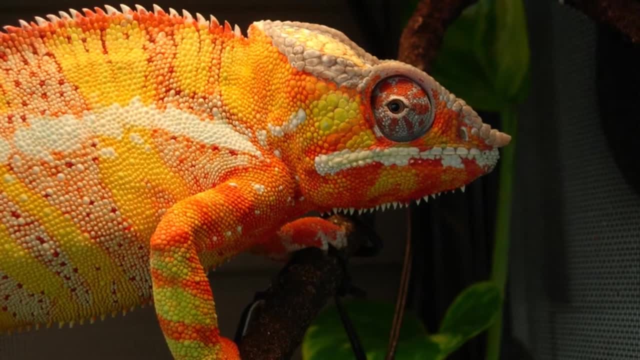 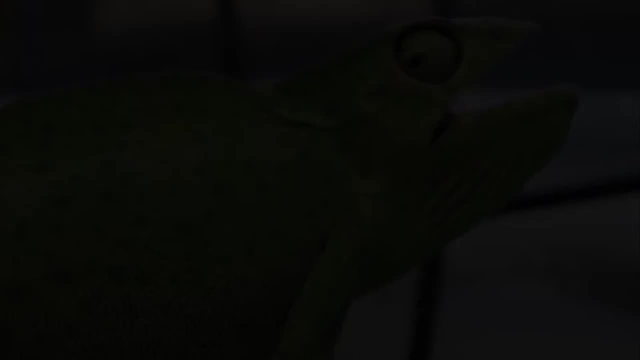 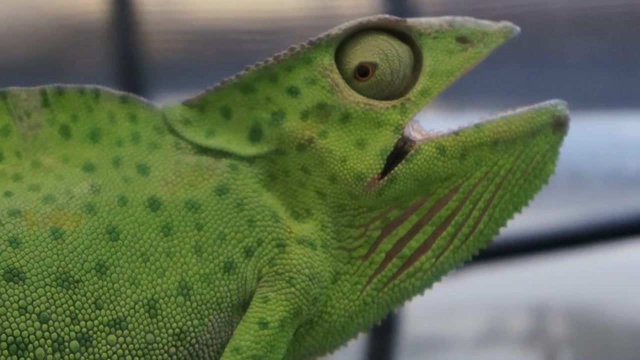 Sunken eyes. Sunken eyes are another tell-tale sign a chameleon is dehydrated. their eyes need plenty of hydration In order to move around and allow them to properly see. if your chameleon is dehydrated, then the eyes will retreat and become sunken in because the skin is not as taut as it should be. this is also a way for them to protect themselves from drying out. 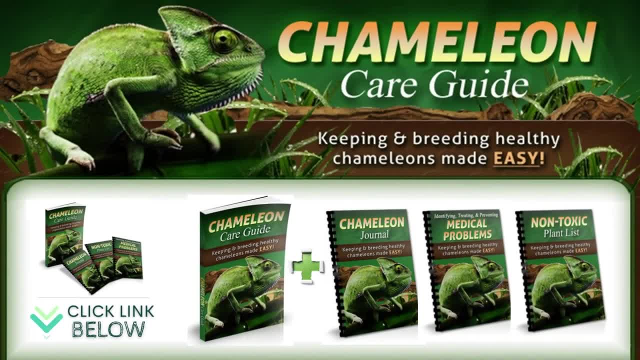 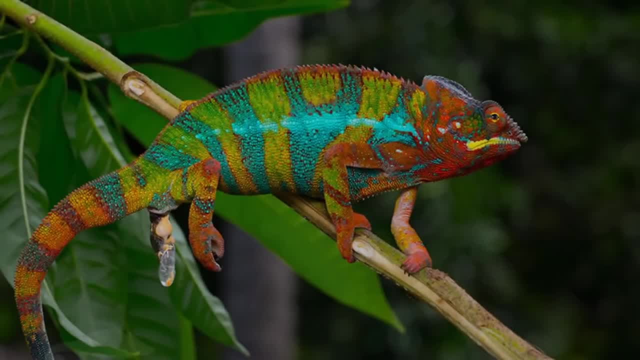 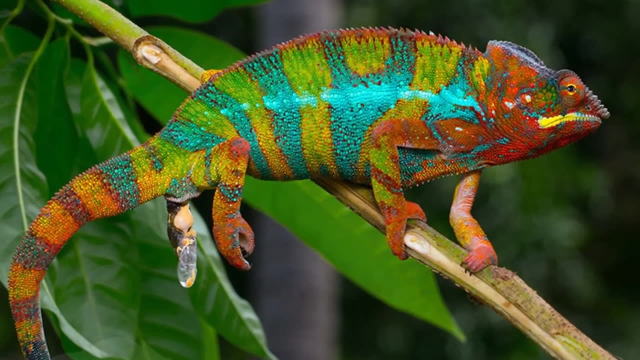 See the chameleon care guide for a detailed explanation of all you need to know about this. I put the official website below in the video description: Yellow to orange urate. Like many other lizards, such as bearded dragons, a chameleon's poop will tell you a lot about its state of health. 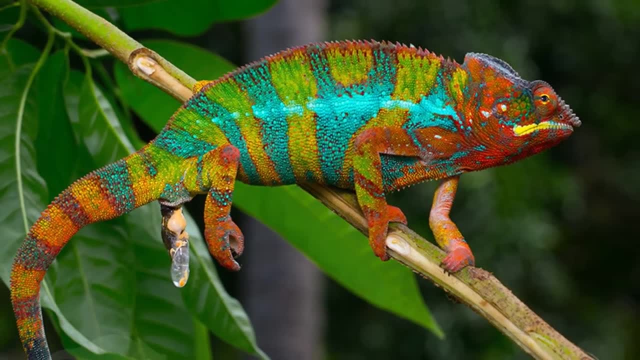 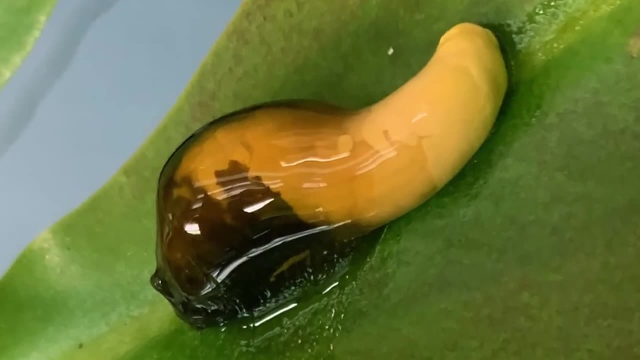 The urate is the white part of their poop. if your chameleon is properly hydrated, then the urate will be white or slightly off-white. however, if your chameleon is dehydrated, then the kidneys cannot produce any white urate. 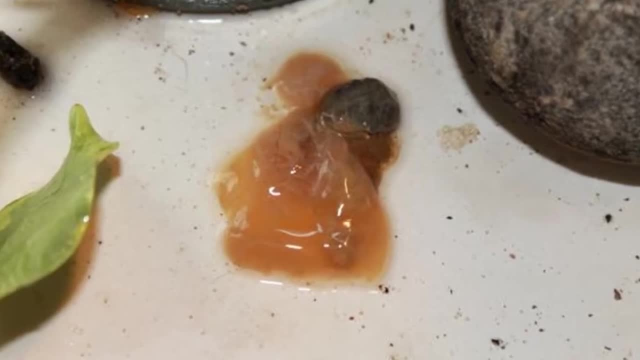 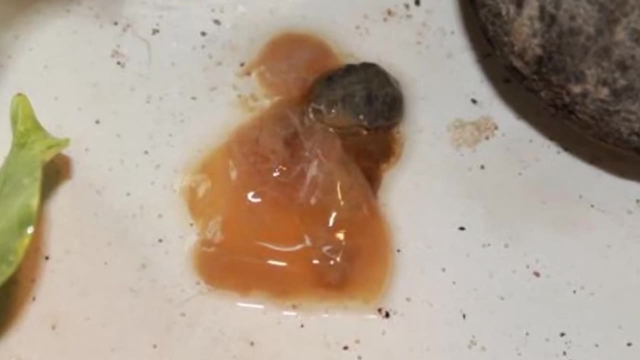 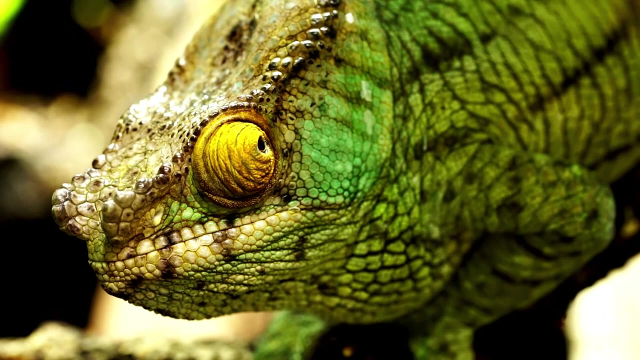 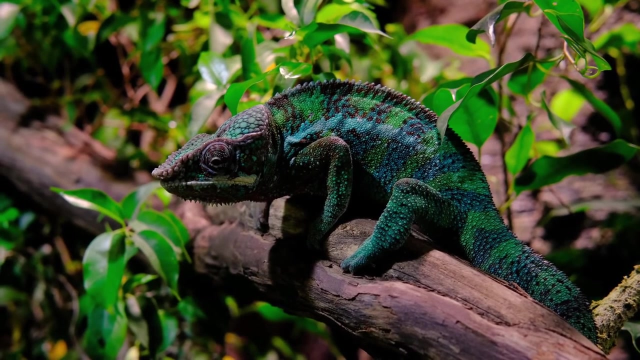 Yellow urate is a sign of mild dehydration or sickness. orange urate is a sign of serious dehydration and you should get your chameleon to the vet immediately if they display the symptom Lethargy. Lethargy means a lack of movement due to fatigue, tiredness or pain. if your chameleon is dehydrated, it will not have the energy to move around as much as it usually does. it might also stick to the lower branches or even the floor of the enclosure, rather than climbing and exploring as they usually do. 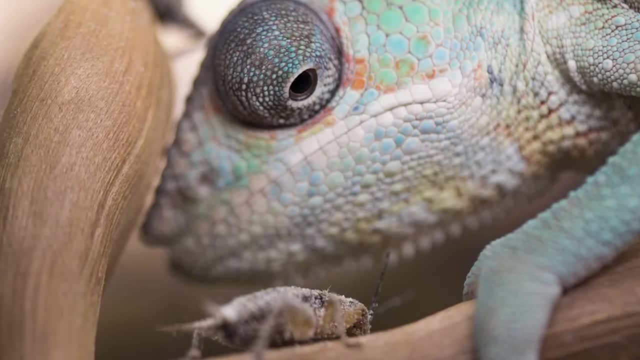 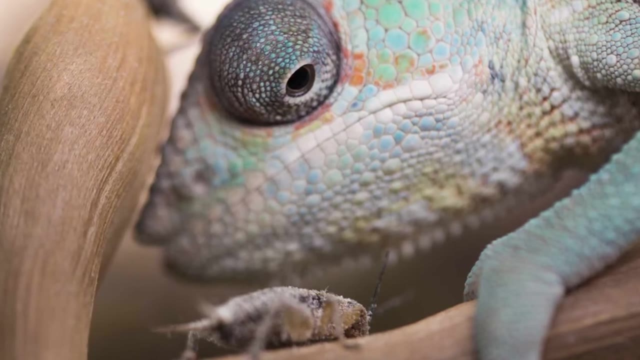 Lack of appetite. A dehydrated chameleon will not have an appetite. this is a problem because food is a key way to reintroduce liquid back into your chameleon chameleon's diet. if your chameleon gets to this stage, you must get them to a vet. 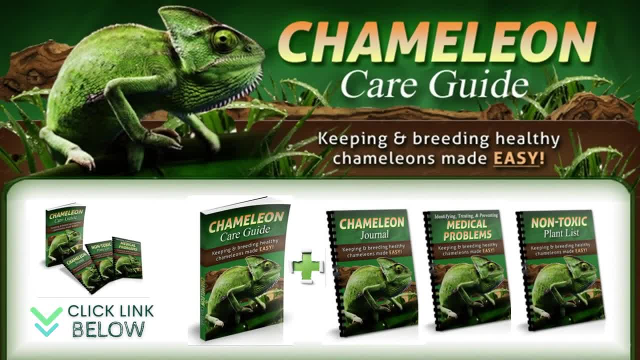 Feel free to download our e-book on chameleon care. it will save you hours and hours of frustrating research and will also eliminate the worries and stress that come with reading something online and not knowing whether to trust it or not. it will also make sure that you do not. 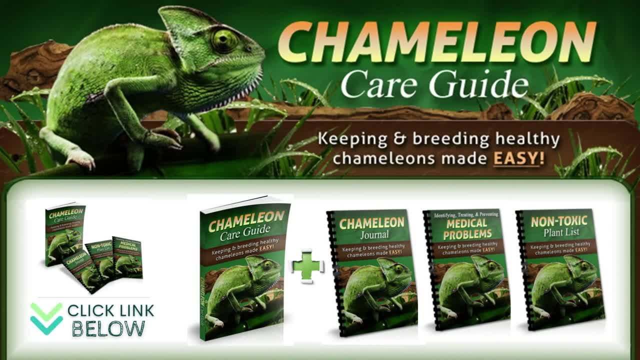 make any mistakes or overlook important facts that could lead to suffering and even death for your pet chameleons. I put the official website below in the video description. thanks for watching.